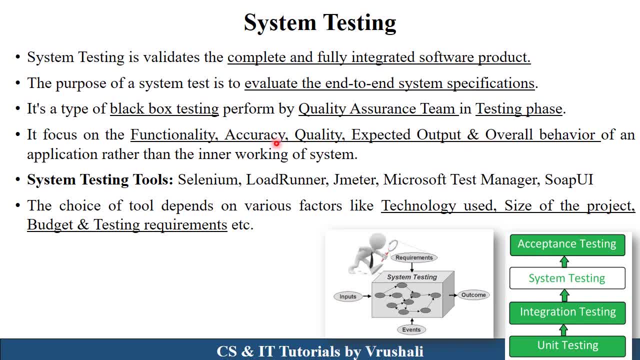 and overall behavior of your product. They test all these parameters. Now in market there are various system tools are available, like selenium loadrunner, jmeter, Microsoft test manager Tester. use those tools for generating different kind of test cases purpose. The choice of the tool depends on which type of technology used in your project. 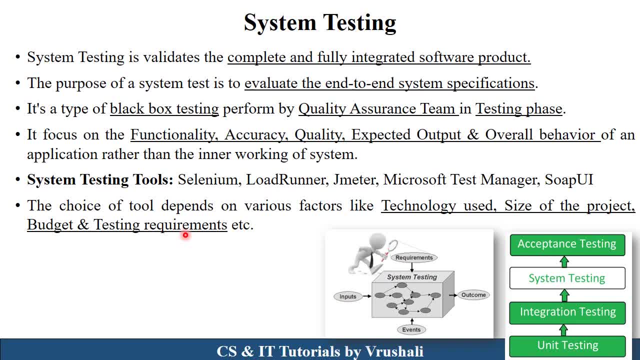 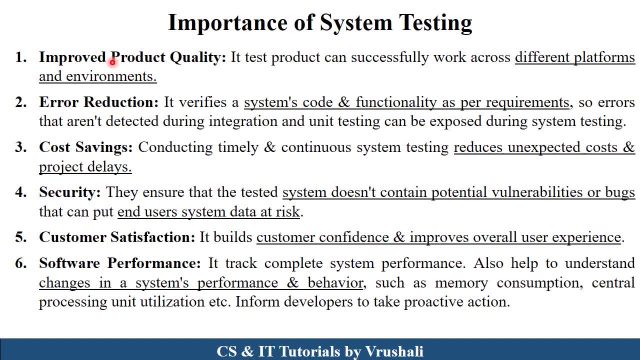 size, budget and testing requirements of your project. Now the next topic is importance of system testing. The main importance is it improve quality of your product. Here tester test that your product is successfully work on different platforms and environment. See, there is there are different types of operating system, like android operating system, windows operating. 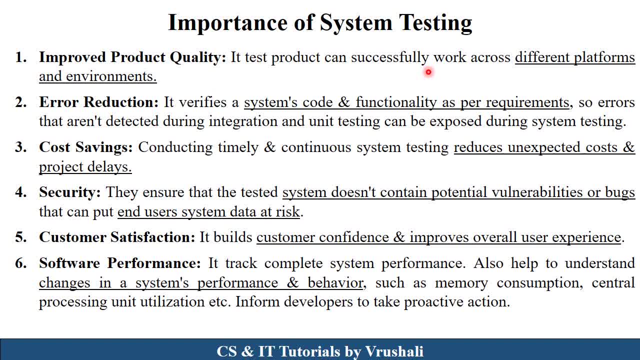 system right, So your product is successfully work on each and every operating system, different platforms and on the customer environments. They ensure all those things. Next one is a error reduction. Whatever the errors are not found in integration and unit testing. these errors are verify in system testing. Next one is a cost saving. Here tester continuously. 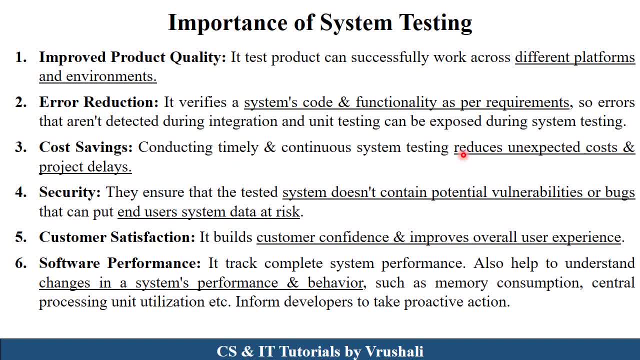 test your product as per the system testing features. That's why they reduce unexpected cost and project delay. The next importance is security. See here tester. ensure that your complete product is bugs free or error free When you deploy your product at the customer environment, so there is no risk at customer. 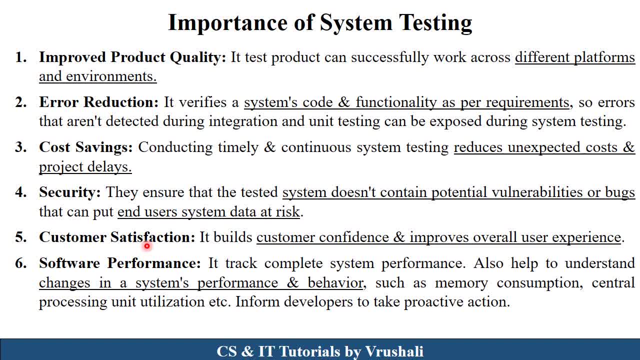 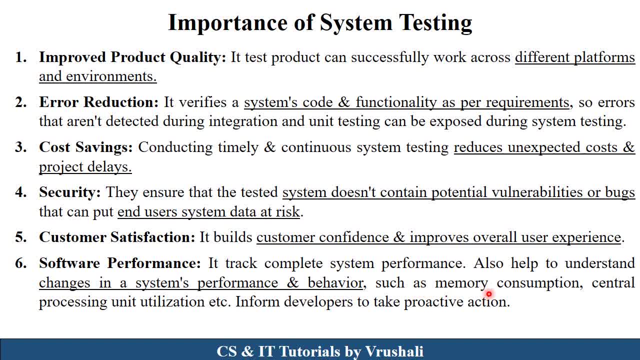 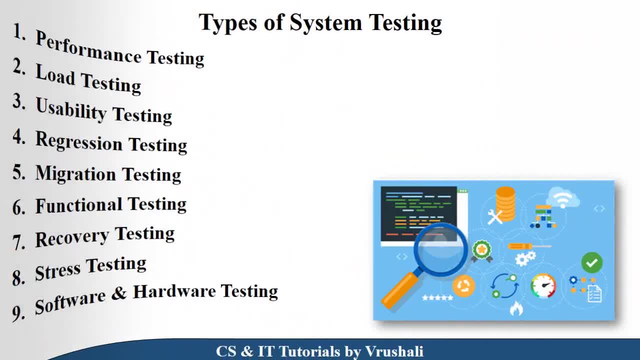 of the product. Here tester test the performance of the productσ chapter title and data flow, in particular product sqrtThere analyze complete memory consumption, processing power, budget, time related to the particular product. Now next important topic is types of system testing. 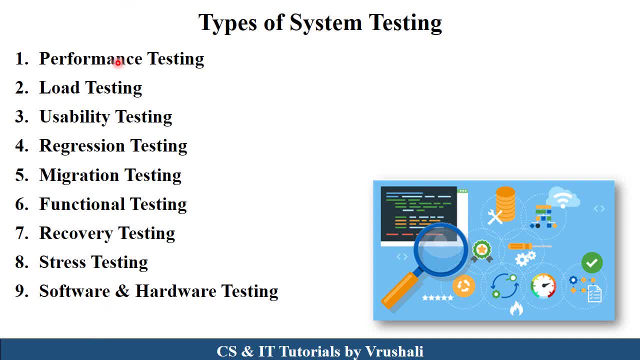 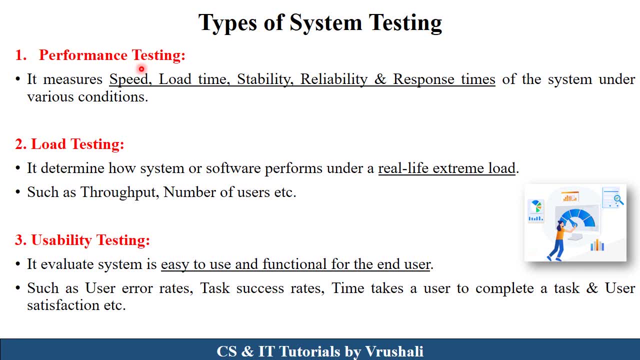 There are total nine types of system testing. Let discuss all these types with example Now. the first type of systems testing is performance testingLet's take a example of You all are familiar with the WhatsApp or any other social applications. When you click on WhatsApp application or the website that will be open within a second right. 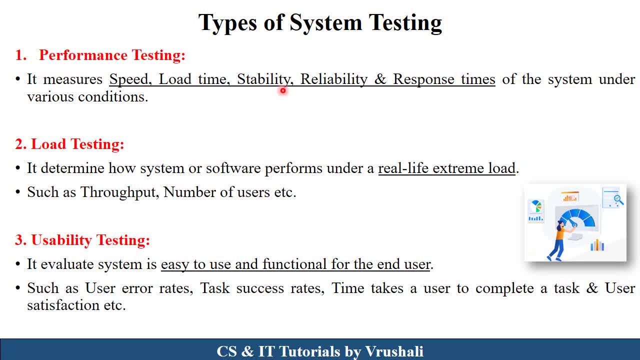 Means they have a good load time and speed. WhatsApp also provide different types of features that will be usable for the customers Means they have a good stability and reliability. You can use different features of WhatsApp like status, audio call, video call at quick time. 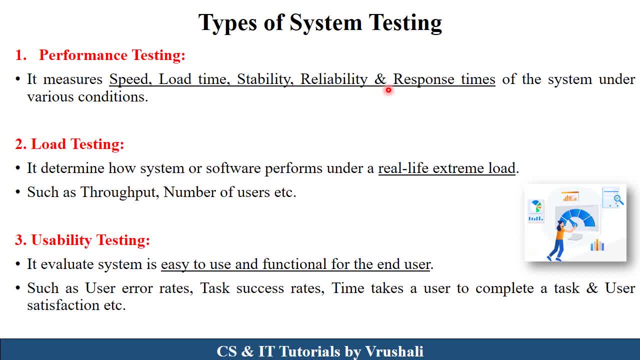 Right Means they have a good response time. So this is called as performance testing. In performance testing they test all these parameters of particular product. Next one is a load testing. See, in load testing they test that your product is work on real life extreme load. 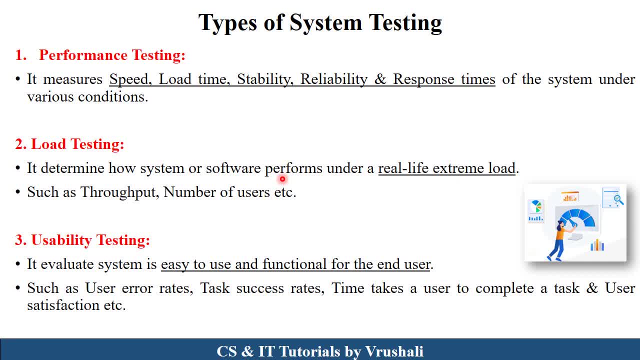 The best example is suppose when your result was declared. At that time all the students are verify or check your result on university website Means there are number of users, number of students are use same website at a same time. So sometimes what happen? the particular website get hang or work slowly, right? 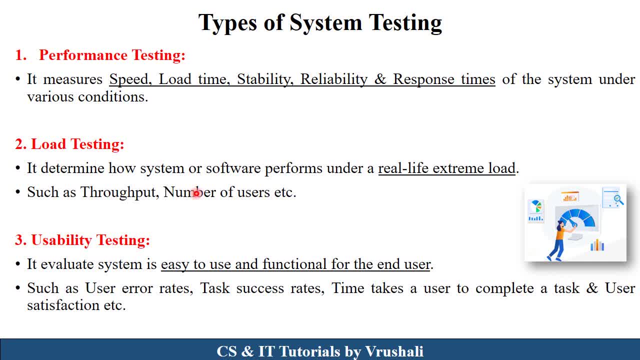 Means their load testing is fail at that time. Suppose there are various shopping application like Flipkart, Amazon, and multiple user use those application at the same time, But still their accuracy, their load, is very good, right? So this is called as load testing. 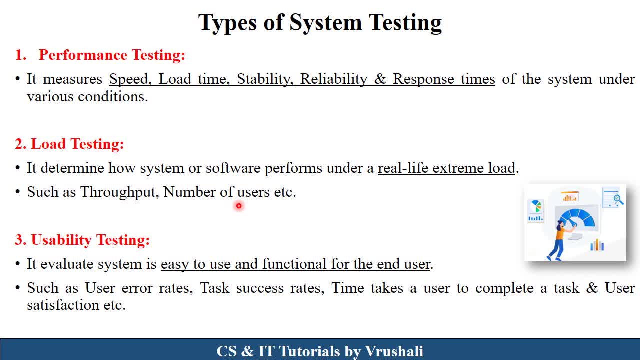 They test throughput and number of users related to the particular application. Next one is a usability testing. The name suggest that your tester test that your application, your product, is easy to use, they provide good functionality and features as per the customer requirements or that will be usable for each and every users. 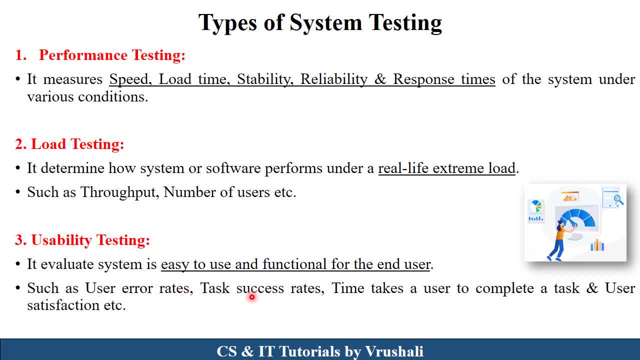 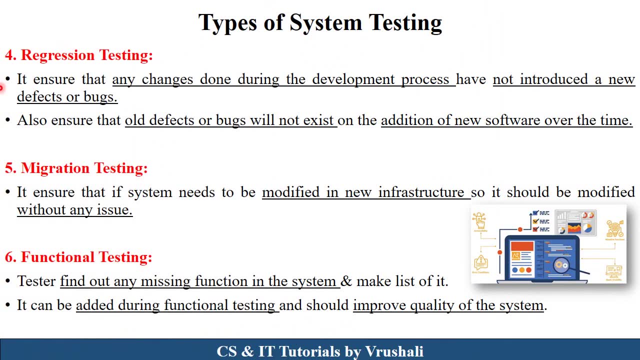 Basically they test user error rate, task success rate and how much time required for completing a particular task task. In usability testing, the main aim is they test that user satisfaction or not related to the particular product. Now the next type is regression testing, As we discussed earlier. sometimes 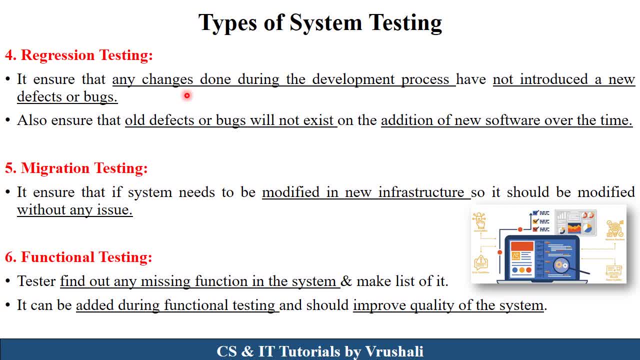 customer requirements are continuously changes related to the particular project. So here, tester, ensure that any changes done during development process which have not introduced any new defects, bugs or errors in your project, So they ensure all that thing- any old defects, old bugs also. 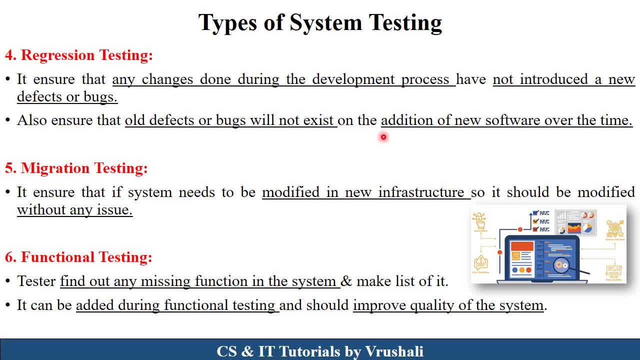 not exist when new features, new requirements will become. So this is called as regression testing. Next one is a migration testing. See, there are different types of updates are available. When you update a particular software or application, then there will be a new features. 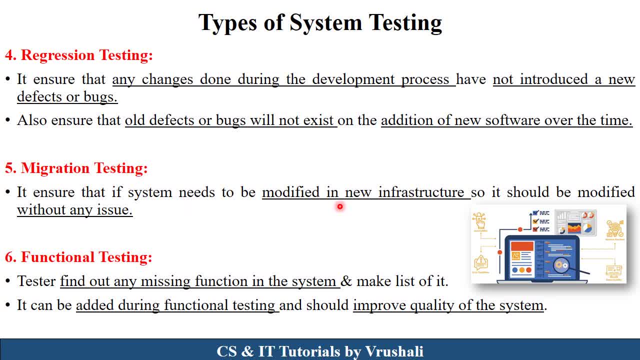 regarding this right. So when you modified a new features, so at that time there will be no any issue related to the particular product or the project. So this is called as migration testing. They ensure that your system needs to be modified in new infrastructure, but it should be. 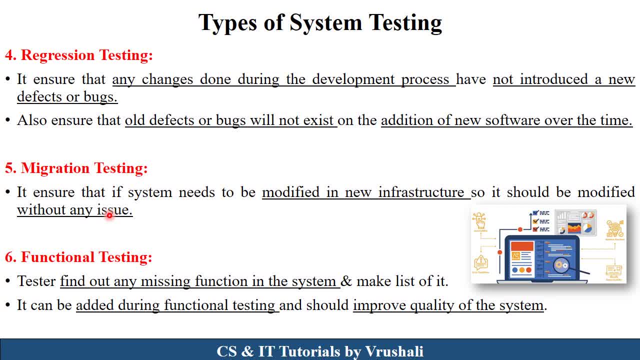 modified without any issue, without any error. The next one is a functional testing Here tester find out any missing function, missing requirements related to the particular system. They make a list of it and send list to the developer. So basically, they make a list of it and send list to the. 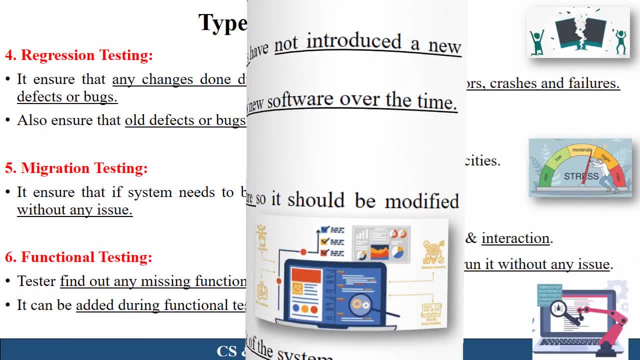 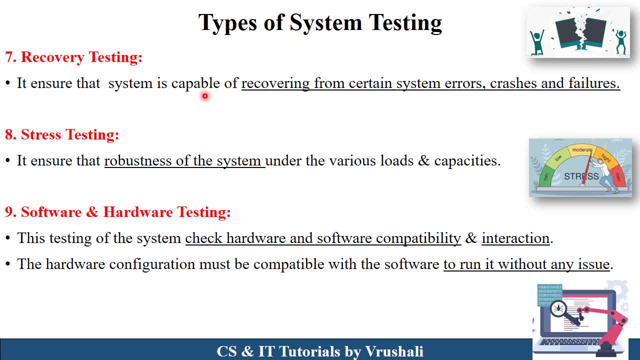 developer. So basically it improve the quality of your system. Now the next type of testing is recovery testing. Here, tester ensure that your system is capable or complete recovery when there is a system error, system crash and system failure. At the time of system crash, there is a no data. 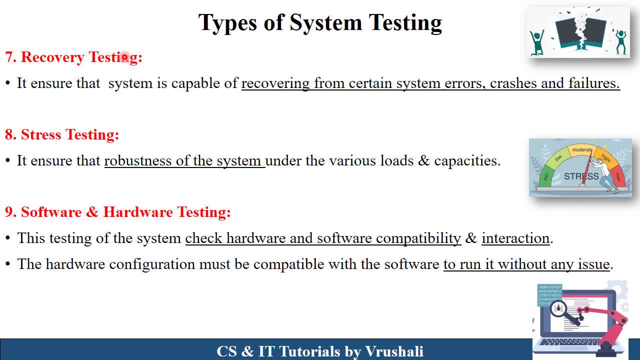 loss. This all things are ensured in recovery testing. Next one is a stress testing. See here in particular project there are various types of load stress, stress, stress, stress stress, stress loads and capacities related to the memory load, then a time bounded load, then capacity load, 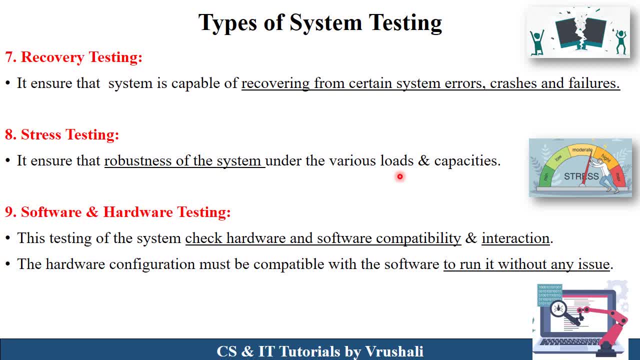 performance load. So when all these loads are happen still, your system is work. robustly means they work accurately and quality result will be generate. So in stress testing tester ensure that robustness of your system. And the last one is a software and hardware testing In your project. 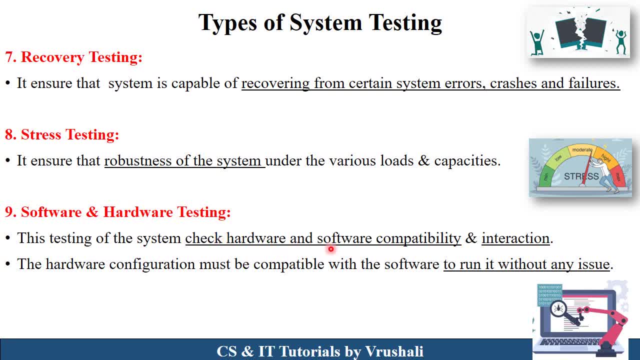 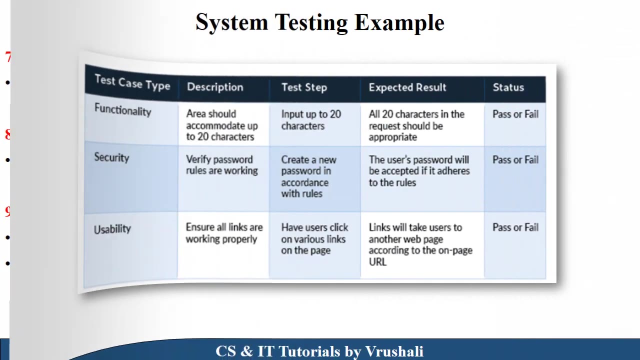 you can use different types of hardware and software devices. So here tester ensure that all these hardware and software particular devices are compatible with each other and there is a good interaction between that, And all these hardware and softwares are run or used without any issue. So this is called as software and hardware testing. Now see here. 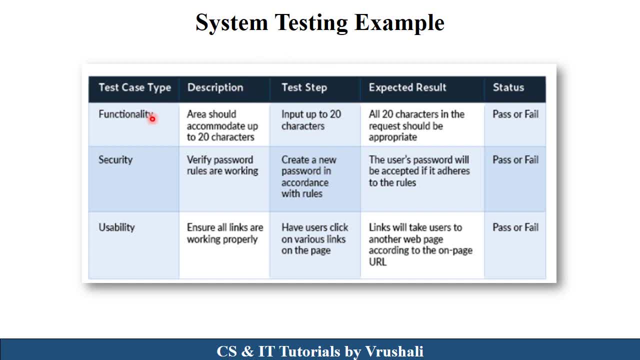 this is just a basic example of system testing. See in particular, registration form. there is a address option, right. So in this case there is a address option right. So in this case there is a and at that particular place there is a text box is given. Now this address contain only 20 characters. 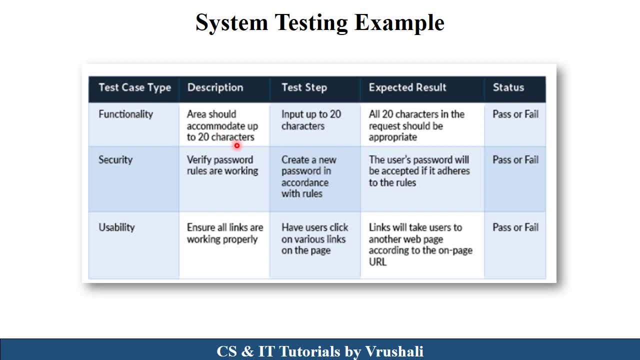 at a time. okay, This is a capacity, that is 20 characters. When user enter more than 20 characters, it display error, right? So this is called as functionality testing. They test functionality and feature of particular component. If it is test is pass, then they generate that you can enter. 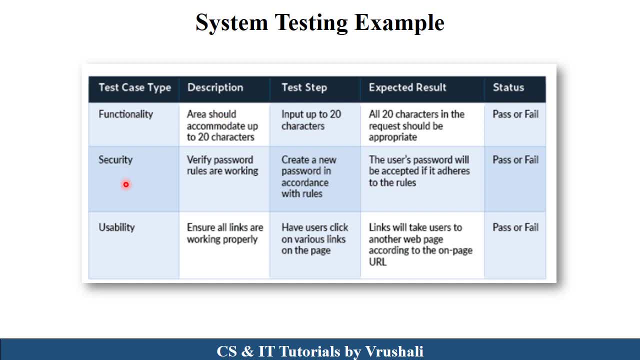 20 characters, in particular address box right. So this is called as functionality testing. So this is called as functionality testing. They are saving application log and transfer data as queue logs, right. The next one is a security. See each and every application. there are user name. 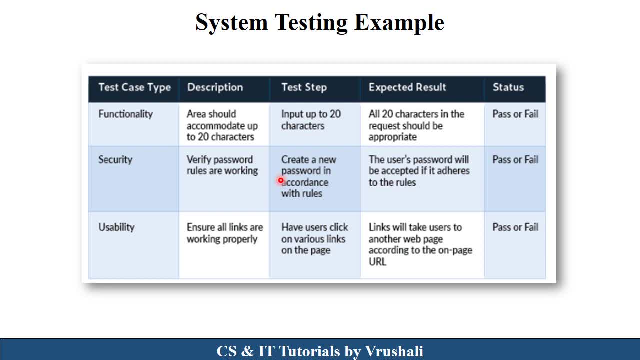 tools like command and password. Sometimes for setting a particular password, there is a control by which your password is set into. For example, if your password is set to 10 or 20,, you can set bekommt to 20,, but when you set the password for every application, there is a. 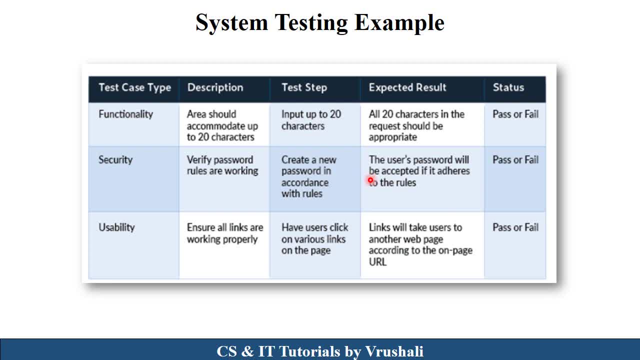 key that tells the user how many characters are already юement automatically. It is also like a ich right. The next one is a tutti security. See each and every application. There is a user name and that time the security testing is pass. but when user does not generate a password, as 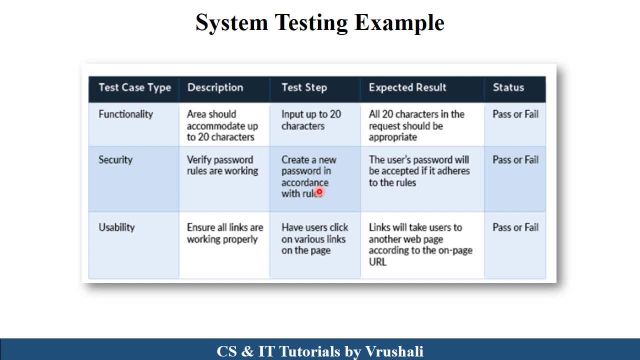 per the rule. suppose user generate only six digit password, so at that time they generate a error and your security testing is fail. and last one is a usability see. in particular website there are various links are available. when you click on link the next page will be open, right? so in usability testing, test those things that each and every websites.